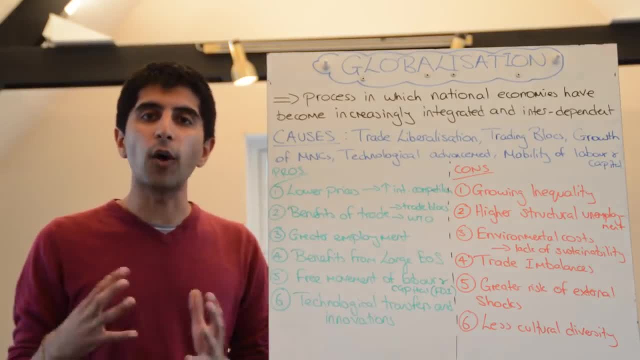 closer together. Interdependent, meaning countries are more reliant on each other, now for growth, for development. So what has actually led to globalisation taking place? It's a phenomenon that we've experienced over the last 40, 50 years. What have been some of the factors? 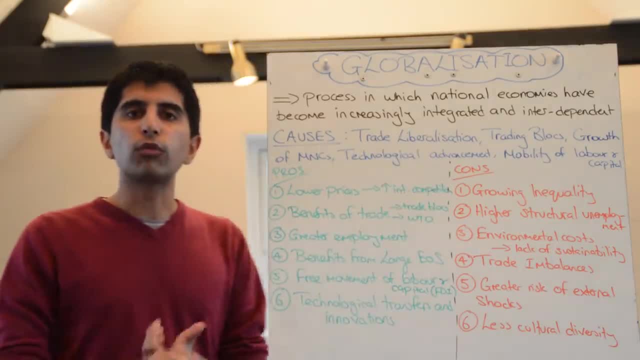 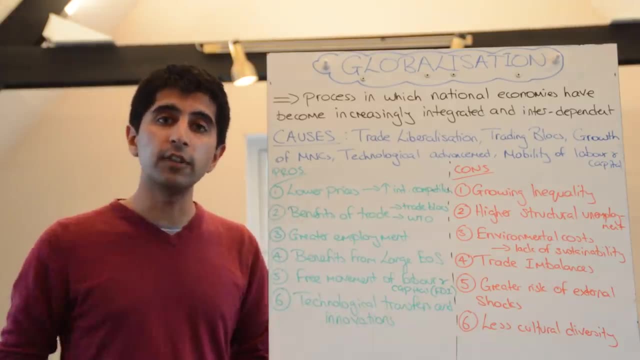 that have led to it? Well, trade liberalisation through the greater role of the World Trade Organisation, through more countries signing up to the World Trade Organisation. It's led to trade barriers actually reducing. It's led to more free trade taking place between nations With more trading blocks. 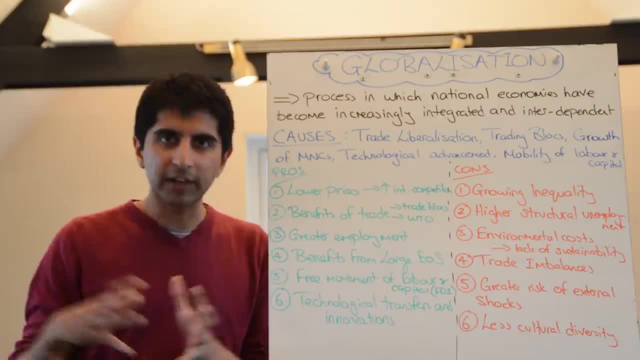 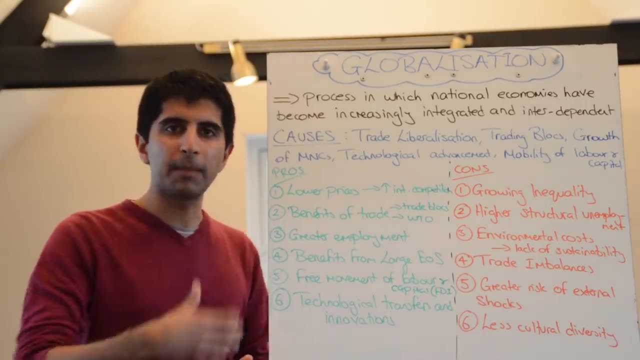 and deeper trading blocks. actually out there in the world again, countries have actually joined together and have integrated. in that respect, In the last 10 years there's been a boom in the number of free trade areas out there and free trade pacts being signed by. 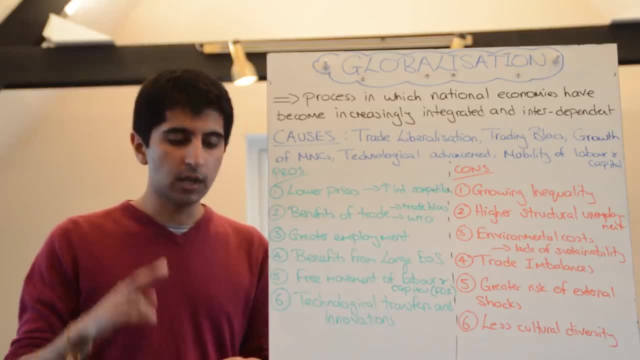 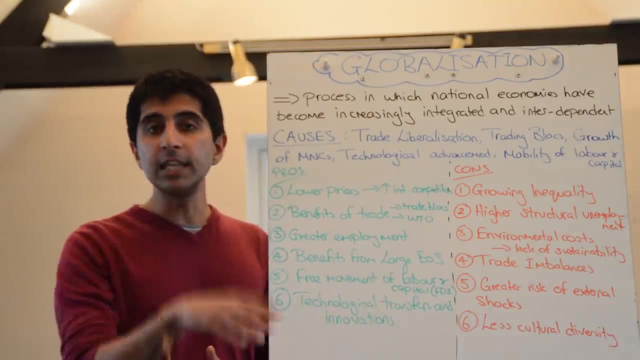 different countries. Right now there are two very good examples I can give you which are on the verge of being completed, which is the TTIP, the Transatlantic Trade and Investment Partnership between the EU and the USA- Again, a big free trade area between the two would be huge- And the TTP- sorry, the TPP. the Trans-Pacific Partnership between lots of different Pacific nations, Again a big free trade area between these nations. The growth of such trading blocks again has brought nations closer together, And even the deepening of existing trading blocks, like the EU, has again meant that nations have become more like one instead of being. 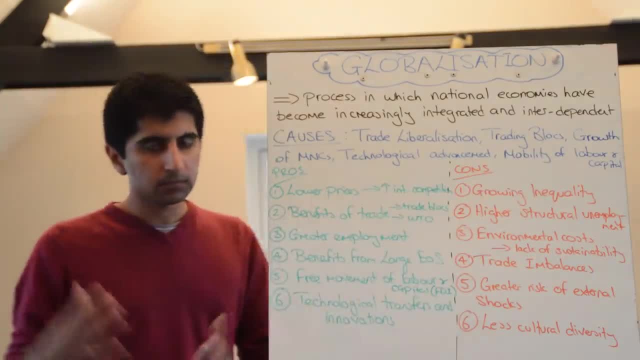 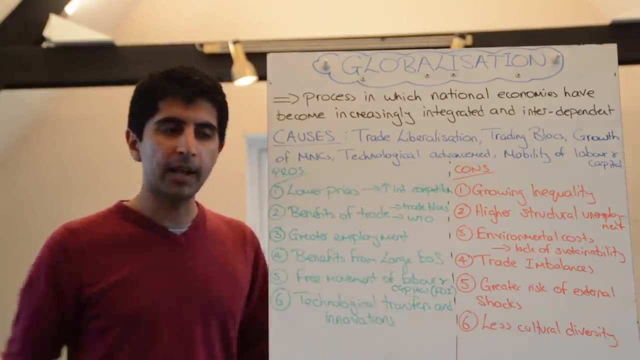 independent. The growth of MNCs- the bigger they've got, the more they've dispersed around the world again- has led to greater integration. We could argue that technology has had a large part to play in that. Technological advancements in the world of transport has made it easier to transport goods and services. 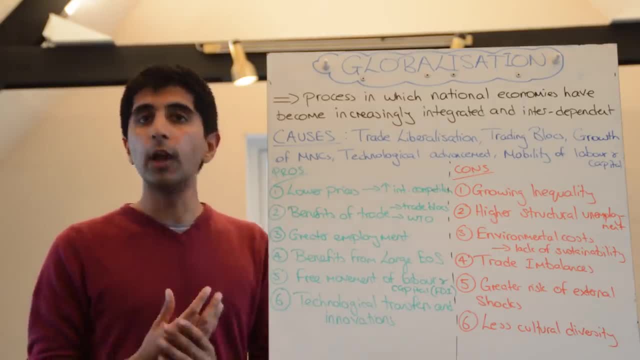 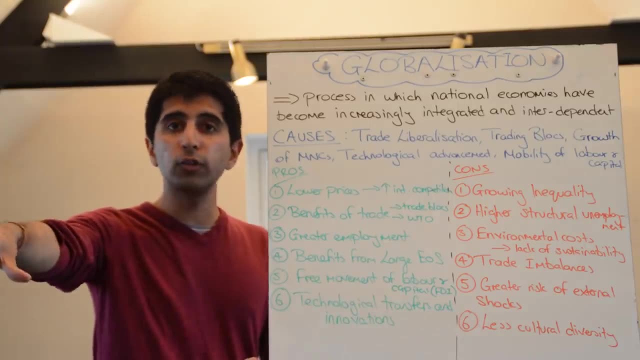 around the world. It's made it easier for businesses to set up in different countries without many major issues. Software development, the growth of the internet again, has made it much easier for businesses, yes, to have headquarters in one country, but still to. 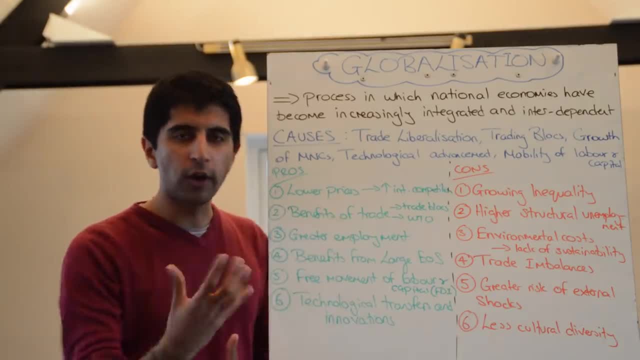 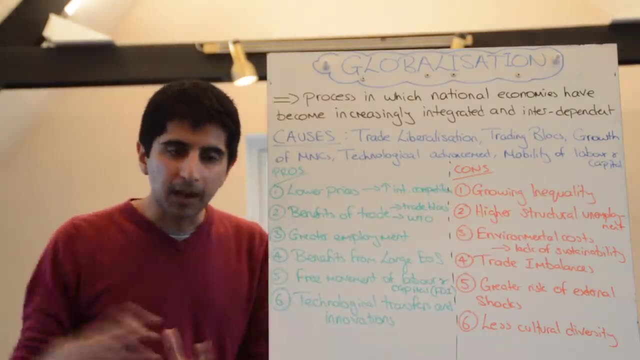 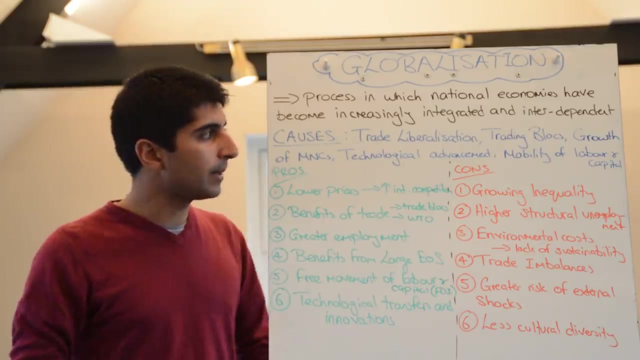 have major outlets at other locations all around the world, which again has integrated the world economy. And finally, with greater mobility of labour and capital, nations are becoming more integrated Again. you could argue that's because of trading blocks, greater depth and existence of trading blocks, but also through government policy, which has 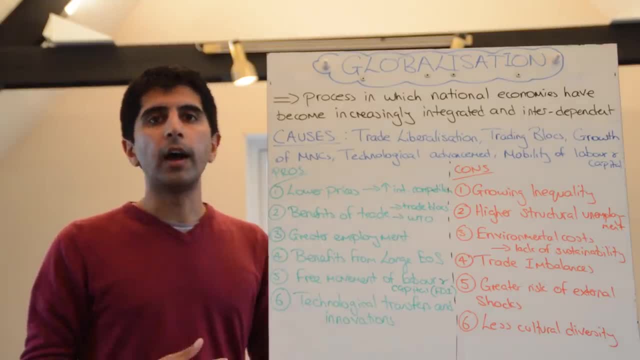 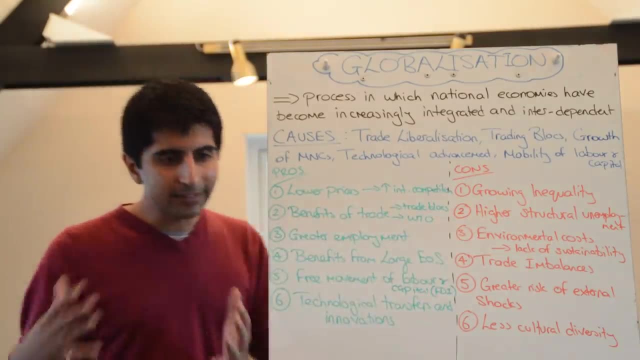 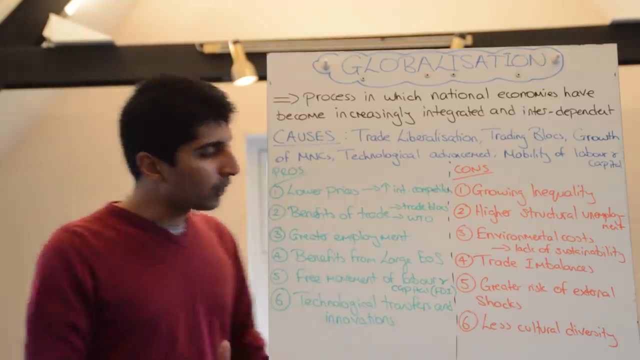 encouraged more migration and the spread of capital around the world. So let's now focus on the pros and the cons of globalisation. Let's understand who's benefited from globalisation and where maybe some economic agents have actually suffered. So what are the benefits? Well, a lot of the benefits come down to great growth. There's a lot of the benefits that come down to great growth. So what are the benefits? Well, a lot of the benefits come down to great growth. There's also smaller profit spirading out towards regionalную. 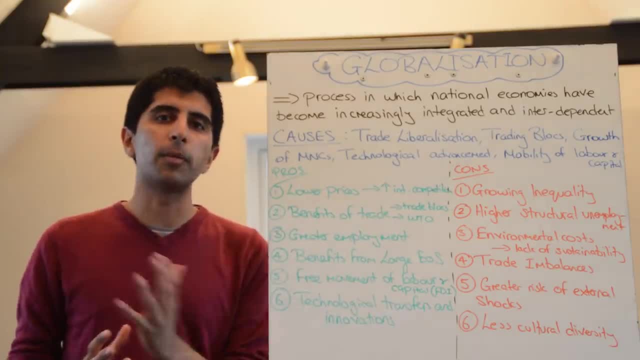 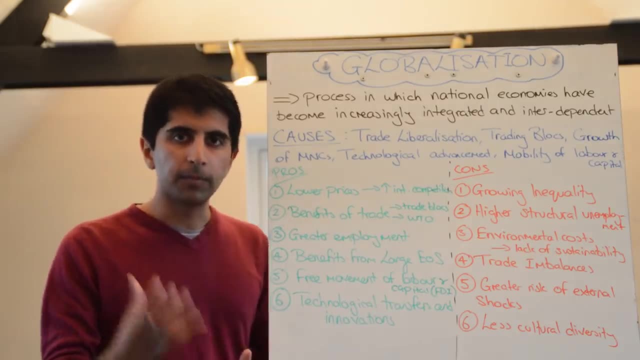 national trade, And it's okay to focus on the trade argument of globalisation. It's a good way to go because there are so many benefits that have accrued from the globalised economy and especially from the benefits of trade that have come from it, So something. 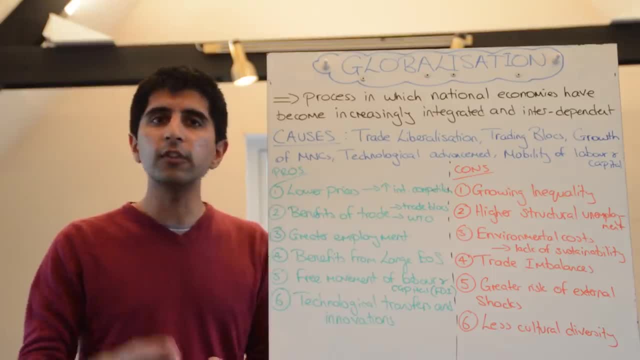 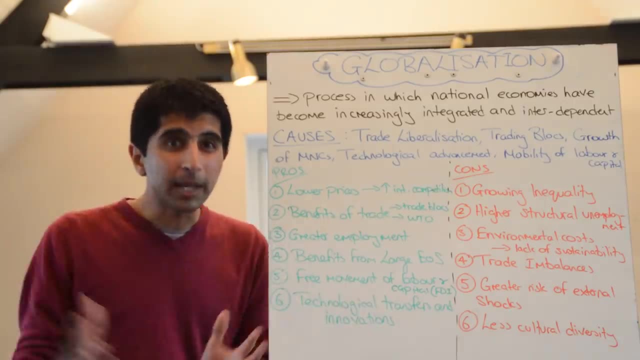 like lower prices. lower prices benefits everyone. It benefits consumers, benefits businesses. This has come from the fact that, as nations have become more integrated, there's is a much, much bigger market. There is more international competition, which puts down the pressure prices, which increases efficiency, lowers costs. Consumers benefit in terms of greater consumer surplus, greater welfare. They benefit from greater market size and market access in terms of more choice of goods and services as well. greater quality of goods and services, more innovative products being developed, more technology- all that kind of jazz they benefit from. But businesses benefit too in terms of being able to access raw materials. 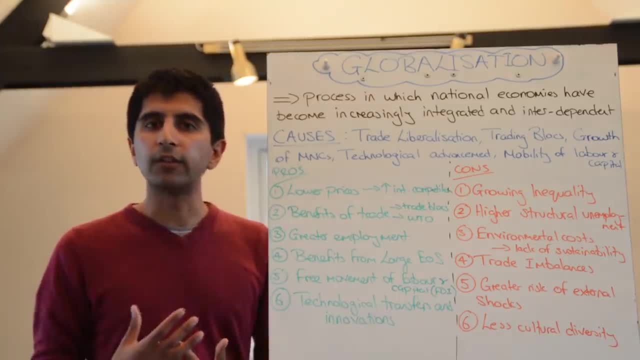 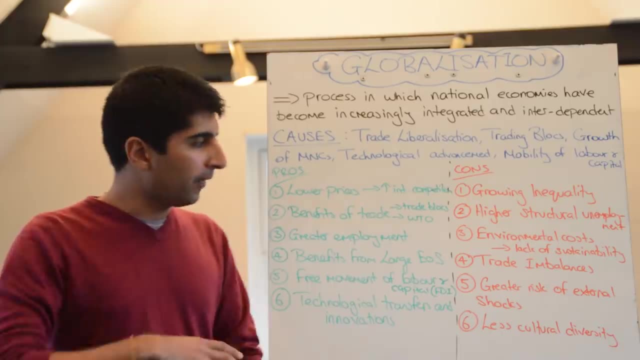 from different given locations and through lower prices, while reducing their costs. It's a big benefit of lower prices right here. Generally, trade has opened up and all the benefits of trade that we kind of know exist have occurred as a result of again deepening 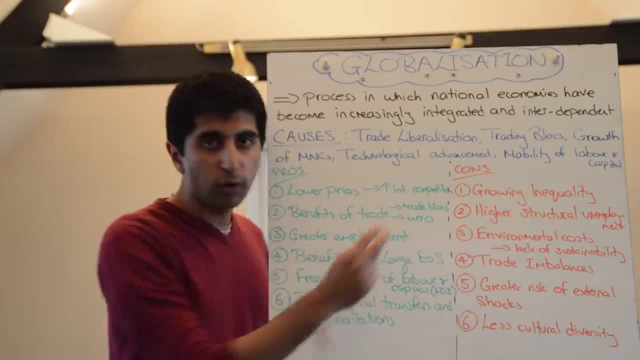 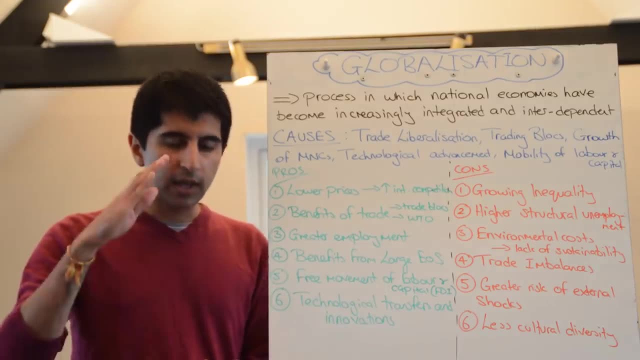 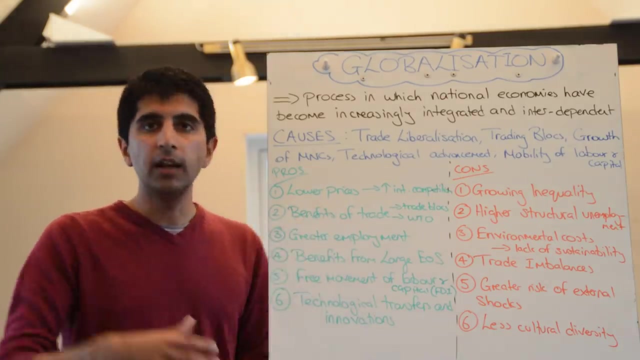 of the trading box and more trading blocks being formed and through the greater role of the World Trade Organisation. So when we talk about the benefits of trade for individual countries, that's been huge Benefits from greater growth, benefiting in terms of governments from greater tax revenues. that have come from the benefits of trade that have come from. greater economic growth For developing countries. their trade benefits have been great in terms of promoting economic development as well. So globalisation, in terms of the trade benefits, have been massive. Let's look more specifically at what some of those trade benefits could have been. So number: three here: greater employment. Again, as the market size gets bigger, as more countries become integrated and are sharing resources and are accessing each other's markets freely, then you can expect firms to grow in size, realising that their potential for trade is. 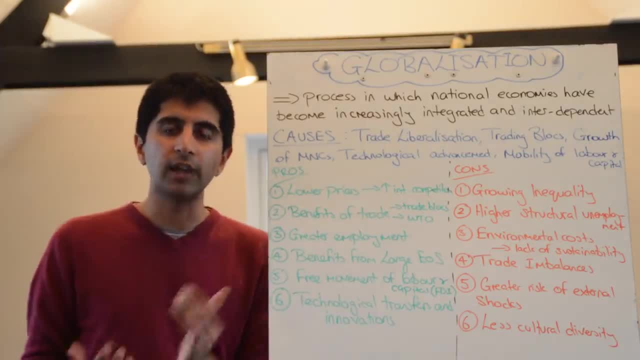 increased massively. The quantities they can produce and sell has increased enormously. What does it mean? It means they need to hire more workers in order to supply that output, which again is great for workers. it's great for individuals who see higher incomes, which means they can. 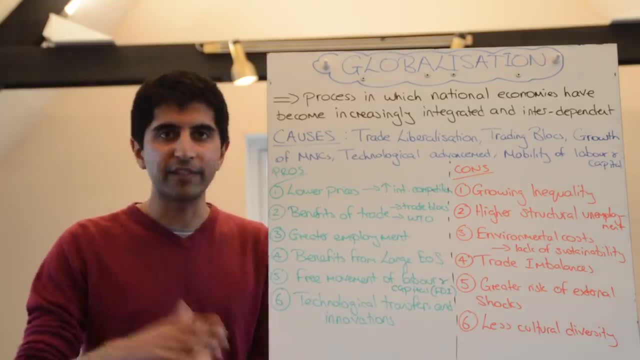 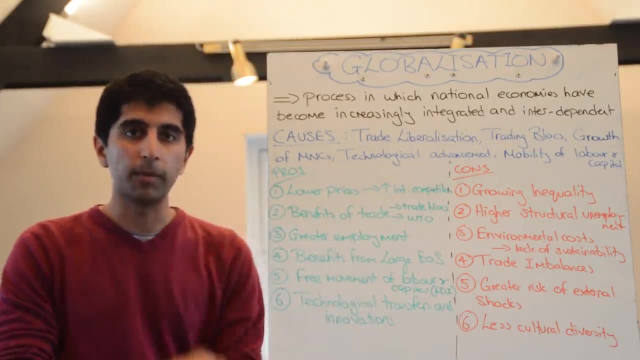 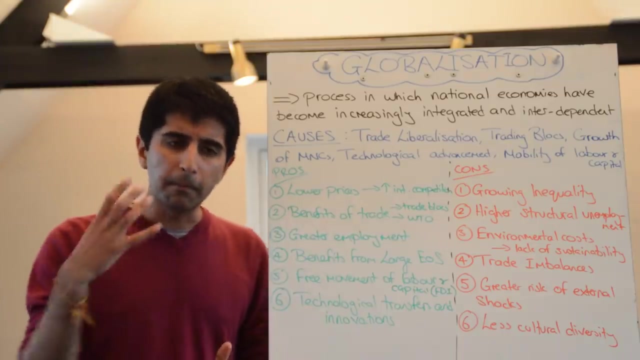 access higher living standards, higher material living standards. they can look after their families more. they can enjoy greater luxury in their lives as a result of it. That all comes from the trade benefits of globalisation here and the employment benefits. Firms benefit from much bigger economies of scale Again as market size gets bigger and bigger and bigger and companies can exploit such size. they can increase their output and lower their costs as a result, which leads them to benefit from higher profits, which maybe can stimulate more investment, more innovation down the road. So that's a huge benefit. right there, Individuals and businesses have benefited from the ease of movement. 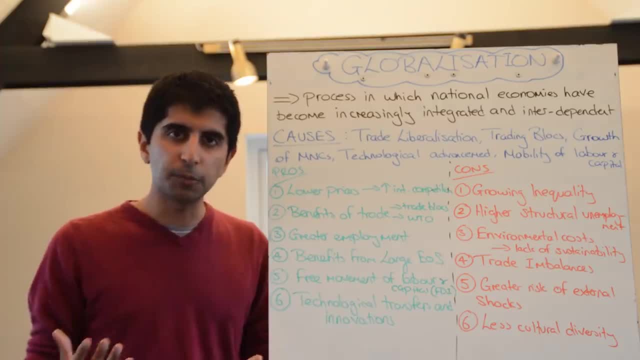 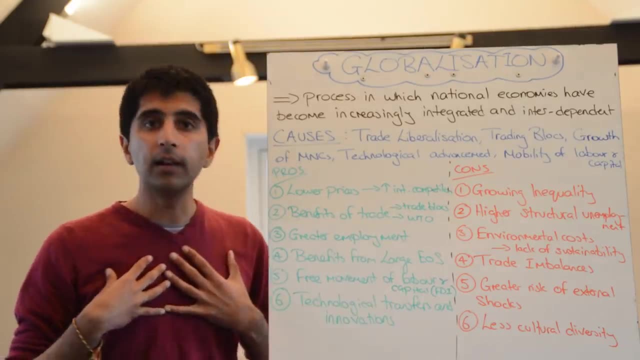 whether that's because of advancements in technology, advancements in transport, or government policy to encourage the development of new technologies. So that's a huge benefit right there. It's a huge benefit to encourage more movement of labour and of business, So individual workers like me I can benefit by being an EU citizen, for example, by the growth of this training. 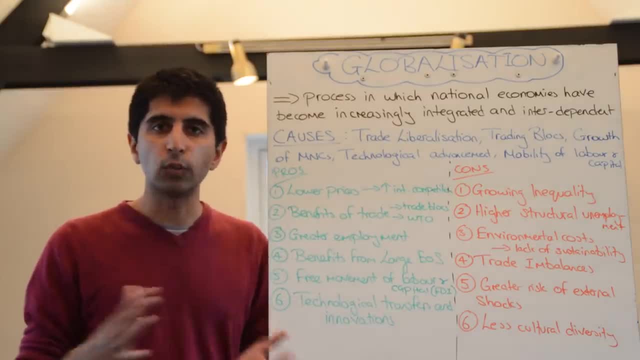 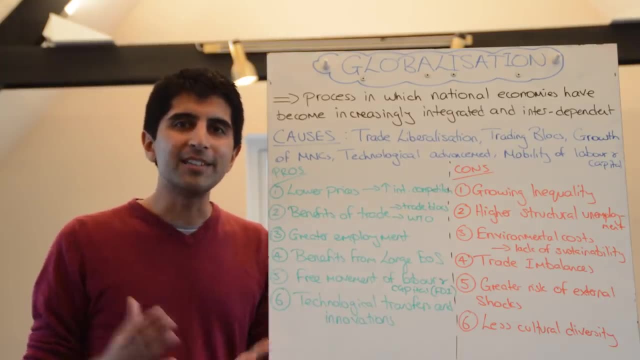 block. I can actually move around the EU completely freely and decide to work wherever I want to, Even internationally. compared to 50, 60 years ago, to move around the world has become much easier. it's become cheaper to actually get visas and to get work permits. 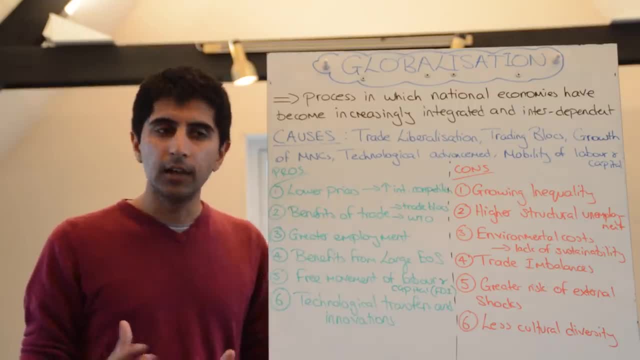 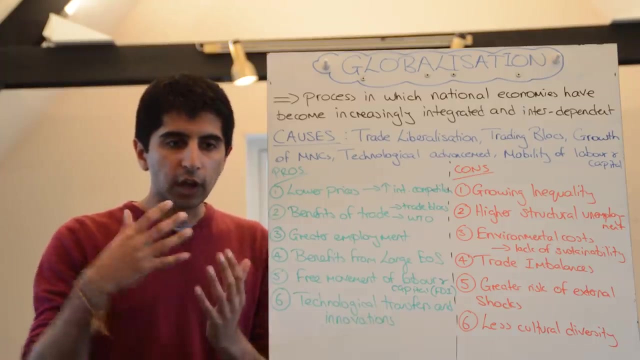 although it's still tricky in some places it has become relatively easier, which again has eased working around the country has made it easier to migrate and therefore migration flows have increased massively recently. But also for businesses to move across the world, for countries to attract foreign investment has become easier through technology advancements. yes, but again through loose government policy which will attract foreign firms to a given nation. And the benefits of FDI are massive for a nation, how it can lead to economic growth in both the short term and the long term for a nation, how it can increase investment. 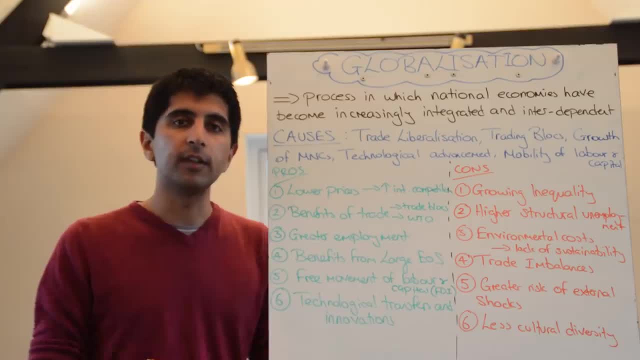 how it can increase investment in the long term for a nation, how it can increase investment in employment, how it can increase profits for all businesses within that country, how technology can actually be advanced through FDI. All these great benefits, the export benefits of FDI as well. So that's been a huge gain through globalisation And I've 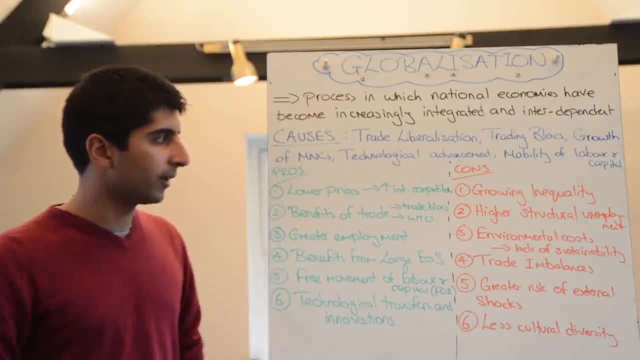 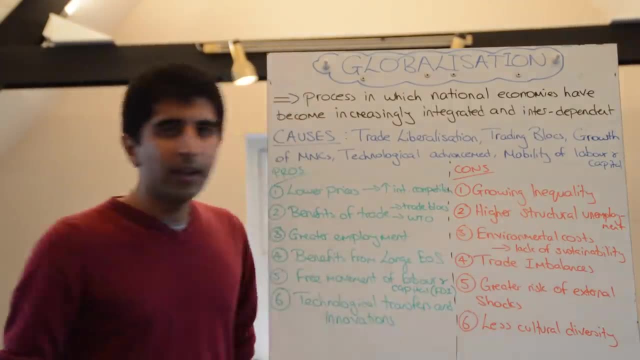 talked about the technological transfers and innovations that have come about through globalisation too, But not everybody is benefited. There are some major arguments against globalisation too, like growing inequality. There's a great study. I read the other day that at the moment 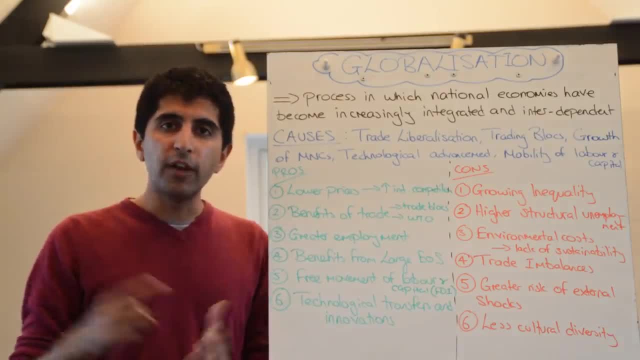 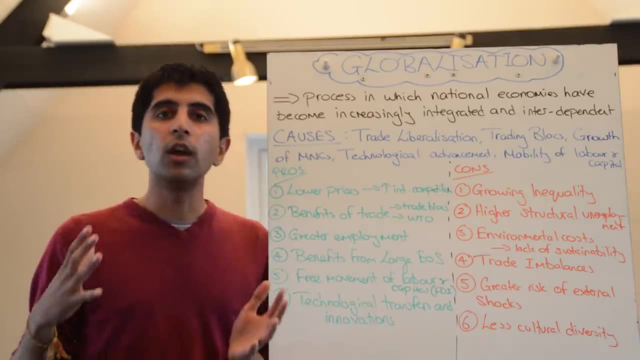 I'm making this video in 2015,. the top 1% of earners in the economy, so the richest 1% of earners in the world economy, own 55% of the total global wealth. I mean, that's a crazy statistic to get your head around And that lets you understand that, even though there have been massive increases in profit, in incomes, in tax revenue collections. this hasn't been spread, for some reason, equally amongst the world's population. Those that have been living in poverty for a long period of time are still not going to be able to. 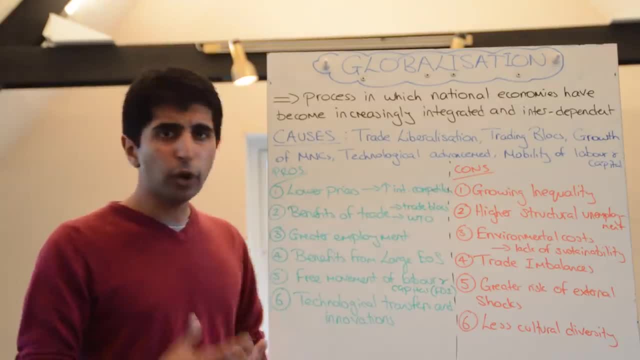 live in poverty for a long period of time are still living in extreme poverty. Those that have struggled and living in relative poverty are struggling to break the class thresholds and to move into higher classes. So there is still this issue of higher incomes actually not translating to higher incomes for all, but just staying to the elite in. 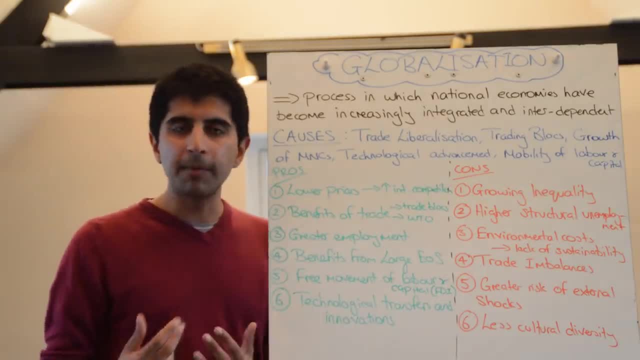 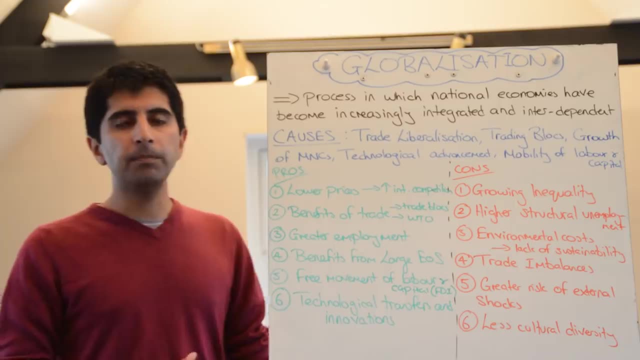 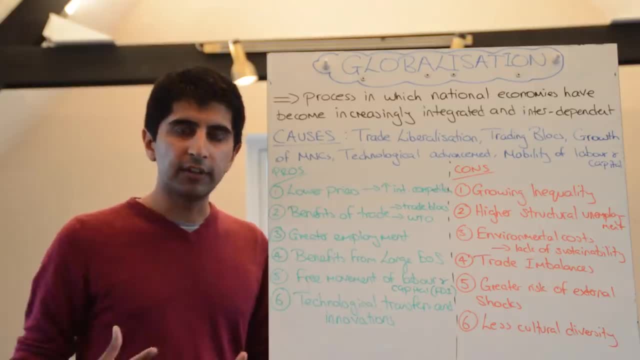 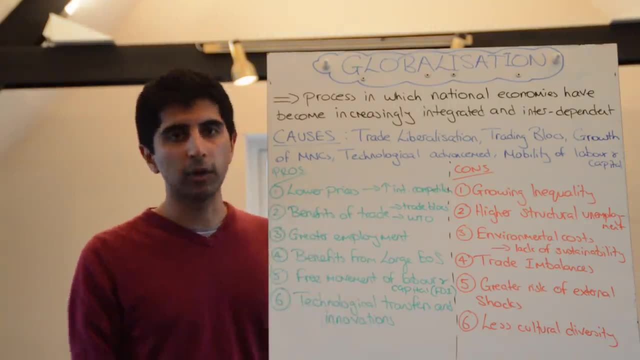 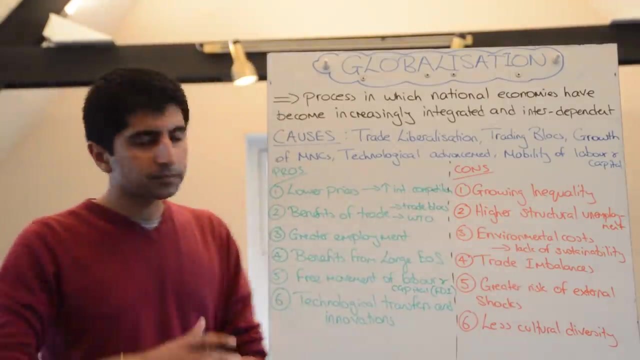 be a greater push for nations and politicians to focus more on alleviating poverty and trying to help those on lower incomes as a result of the gains that come from globalisation, because inequality has grown over the last 20 years or so. If globalisation is taking, 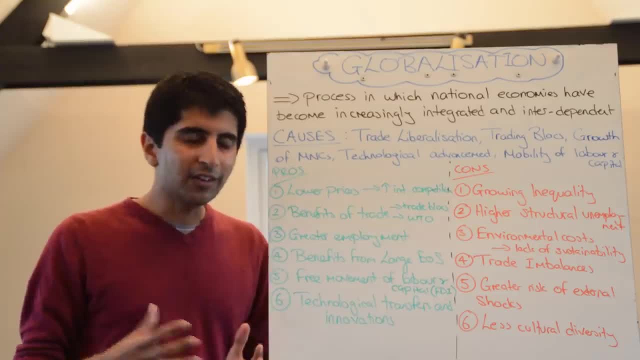 hold at a great pace as well. there is a risk that, as a nation, as you become more integrated with other nations in the world, you struggle to compete. That could lead to businesses going into decline, businesses losing out to international competition, which could 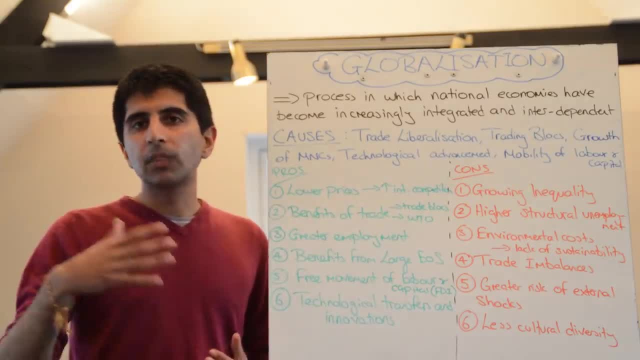 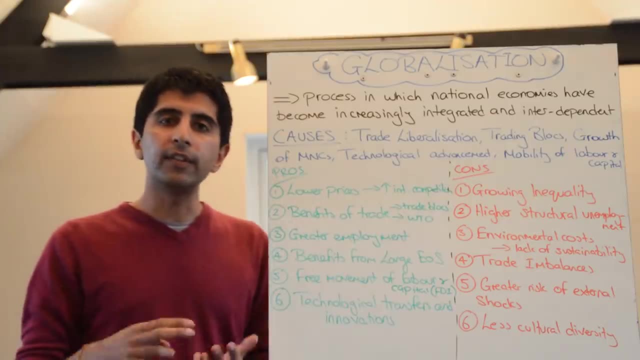 lead to greater structural unemployment, which could lead to people actually losing their jobs, losing their incomes, losing their livelihoods, And in developing countries, that's a major issue- where there isn't the safety net of a strong welfare state, That's a big issue. 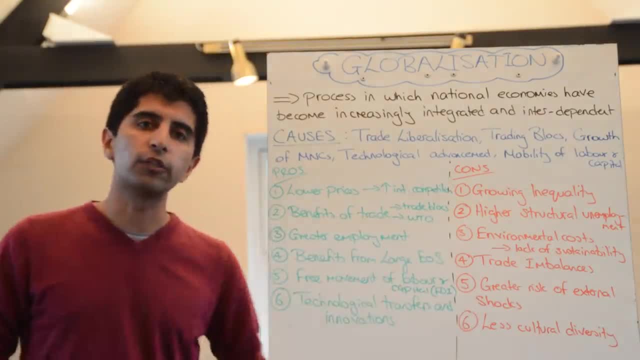 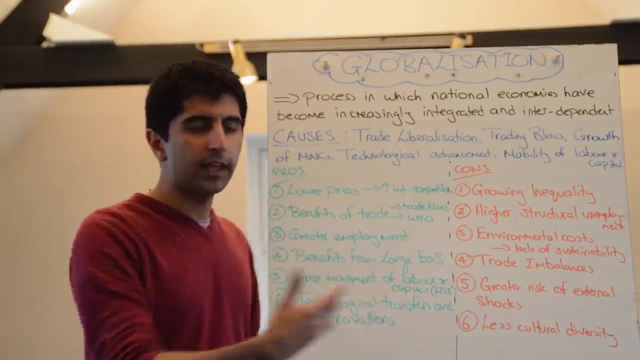 Number three is a massive point as well when we talk about the environmental costs of globalisation. What's been at the forefront of politicians' minds over the last 40 years, as globalisation has taken hold, is the fact that there is a need for globalisation. There is a need for 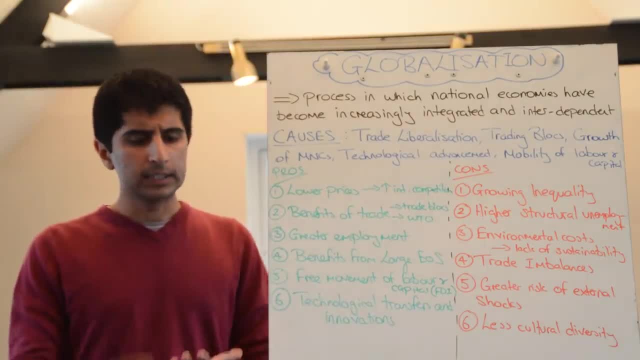 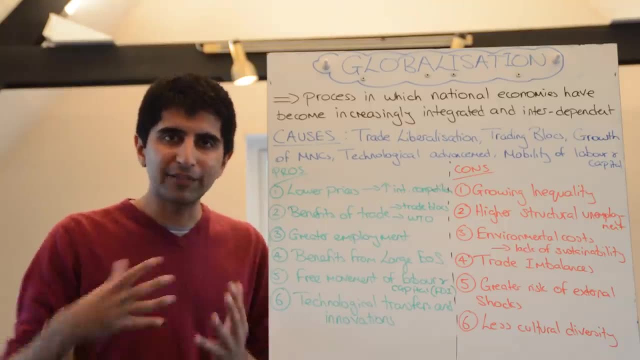 globalisation, There is not just more growth, putting growth ahead of everything else, And what that's meant is that there is a bit more pollution in the world As foreign firms have come and invested, they've taken advantage of resources and they've depleted resources. 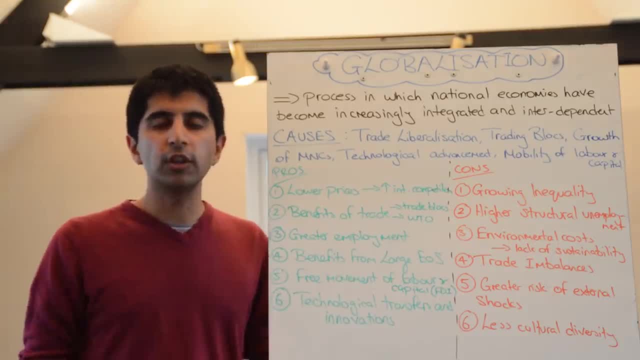 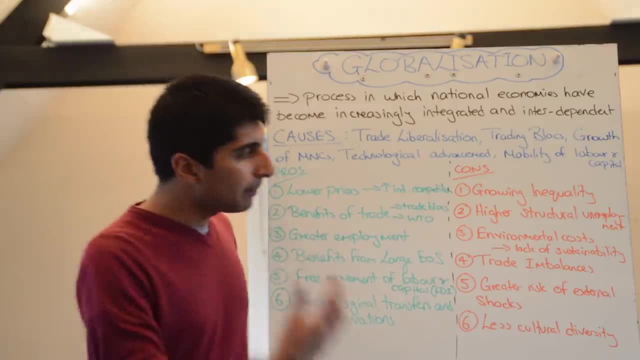 Firms have degraded resources in order to grow, in order to produce. They've degraded natural resources like rivers and lakes in order to produce, dumping waste in valuable resources, And what that means is future generations will suffer. They're not going to accrue the 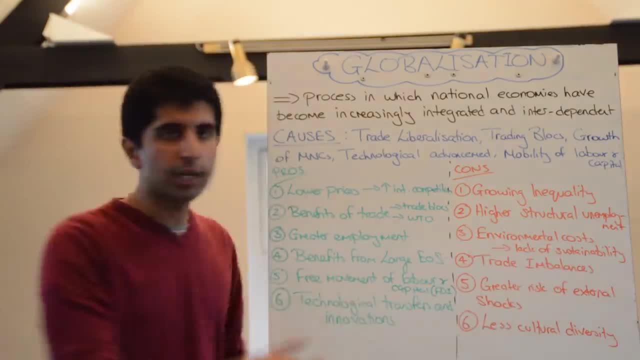 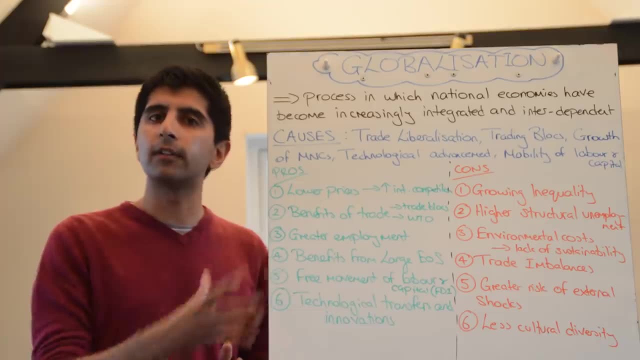 same benefits that we are currently. There is a lack of sustainability in growing in that way, So again, the costs to the environment significantly outweigh, you could argue, some of the benefits that have accrued from globalisation. Trade imbalances as well. The more globalisation has taken hold, the more countries have realised 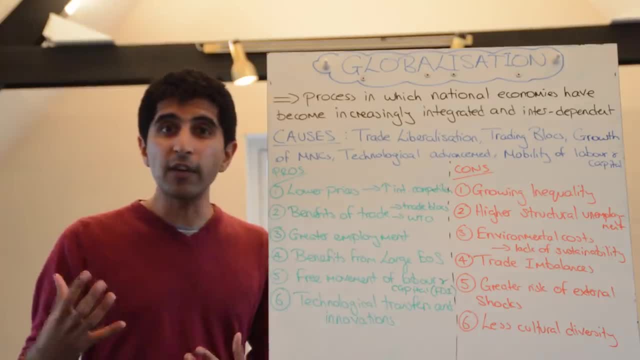 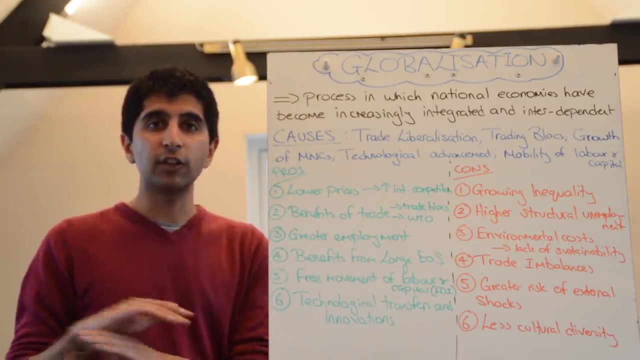 that relying on export-led growth could actually be a very, very lucrative way of growing and developing. Look at China, for example. They've realised the massive export gains as a result of a more integrated and globalised world economy. What it means is if, for some reason, this avenue of growth actually slows down or there is. 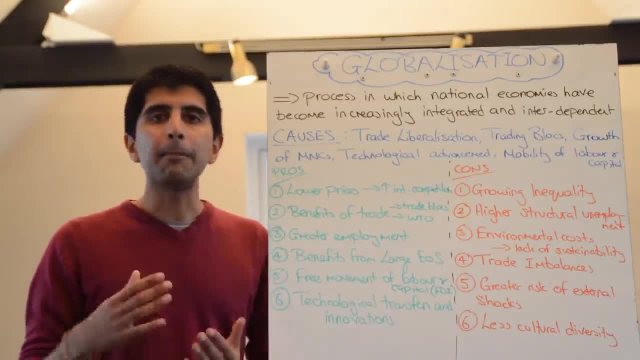 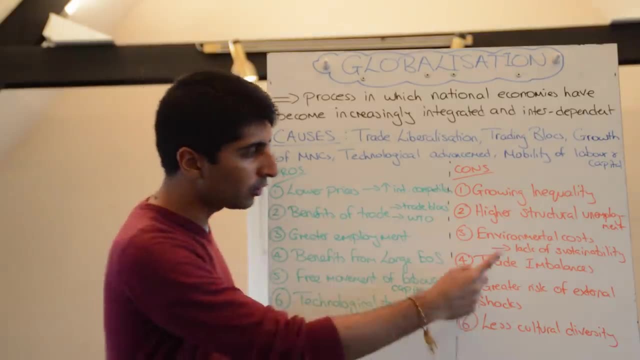 a shock that actually limits the growth potential from exports. it might lead to more protectionist activity and trade wars developing in order to rectify such trade imbalances. So when we talk about trade imbalances we mean things like current account deficits and current 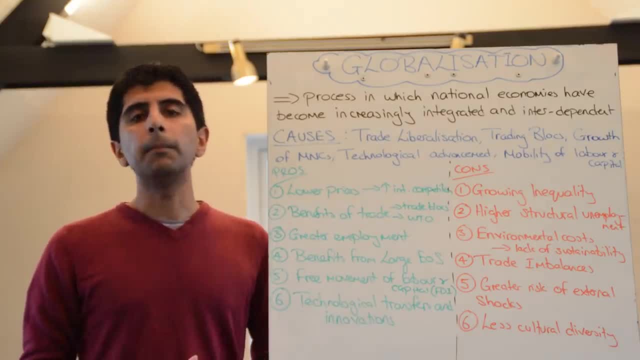 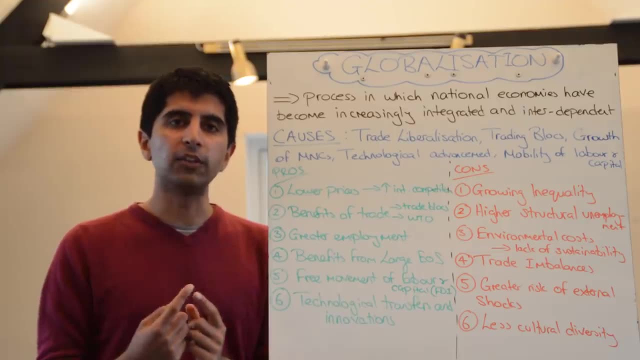 account surpluses. You see more imbalances as such, which could lead to protectionist policies, trade protectionist policies being used far more and trade wars between those countries, nations actually distorting some of the gains of globalization and of trade. There is a 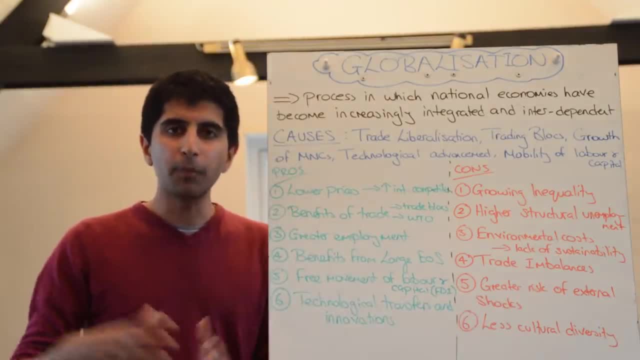 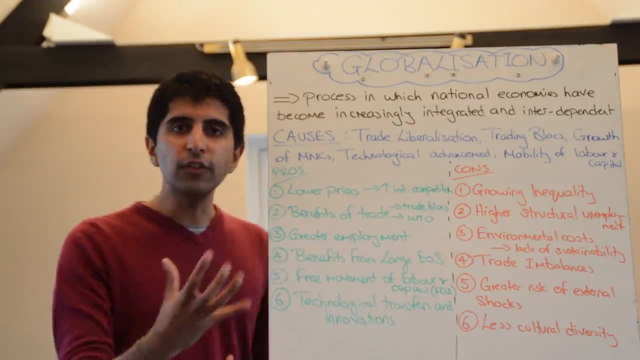 greater risk of external shocks as countries become one, basically more integrated. If one country goes down, they could well take down another country too, And in fact, not just a country goes down If a given industry has a shock or goes into crisis in one nation. 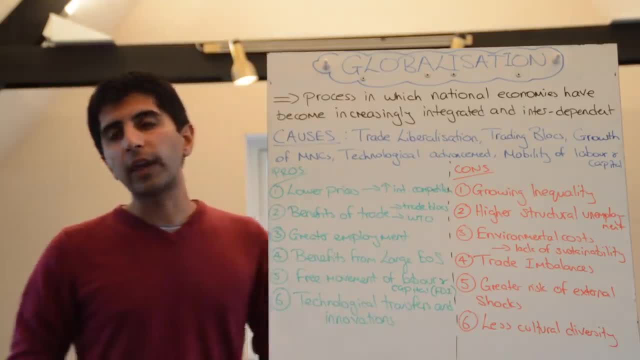 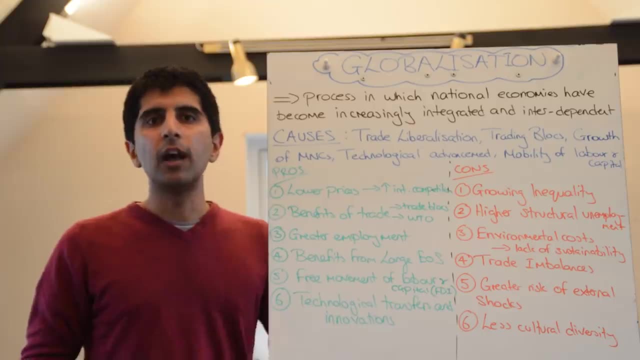 that could spread to other nations around the world. We saw that in 2008,, didn't we? with the great financial crisis? a banking crisis that started in the US, But because banking has become such a worldwide kind of industry now and banks set up in lots. 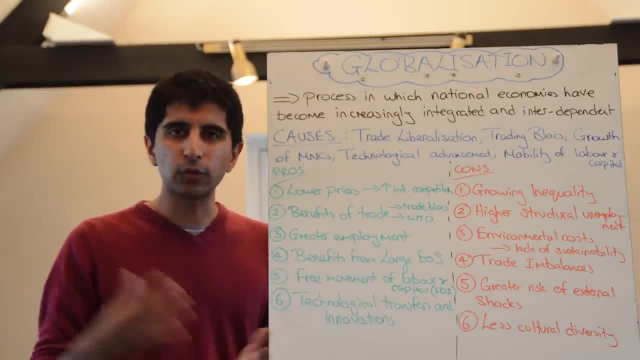 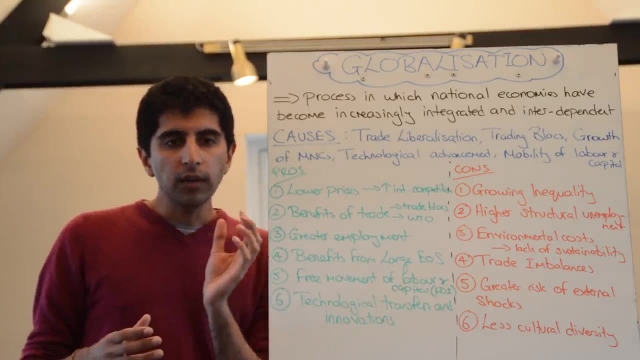 of different countries can be working with billions and billions and billions of pounds of dollars worth of transactions at one time in lots of different nations. one kind of banking crisis in a nation can actually spread all the way around the world. It can take down banking industries in lots of different countries too. What it means is that other 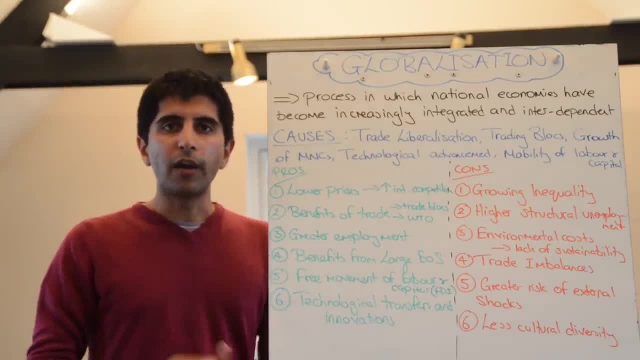 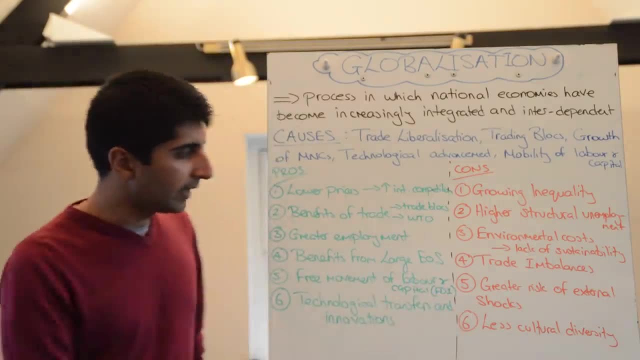 nations are susceptible to massive macroeconomic shocks, are fried down in that sense, and that can lead to deep crises and deep recessions, And we've seen that in 2008.. And also less cultural diversity. This is a big issue as well. If you go to Europe, for example, you'd 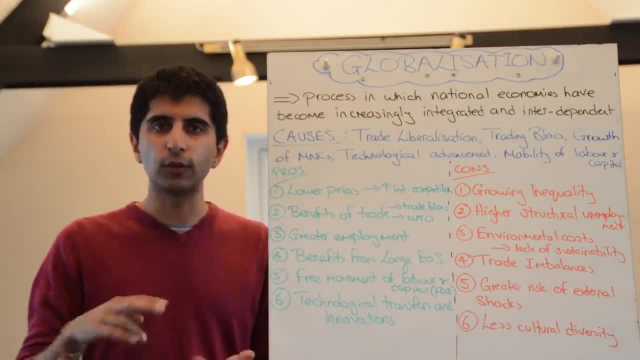 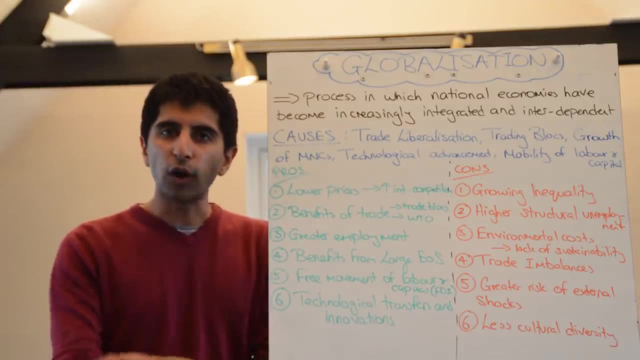 expect if you go into wonderful kind of Spanish cities or Italian cities or Greek cities, you'd expect to see the uniqueness, the cultural diversity that's on show that these countries have to offer. But actually what you'll see are the same kind of outlets, the same kind.